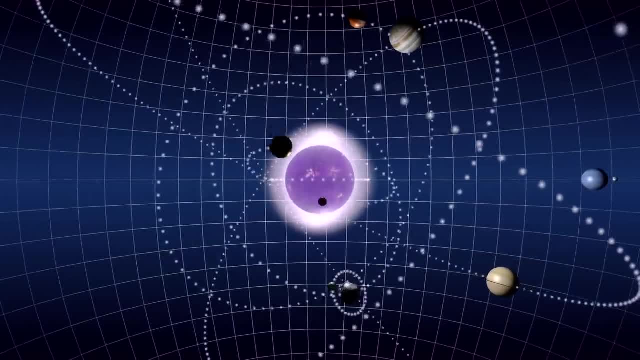 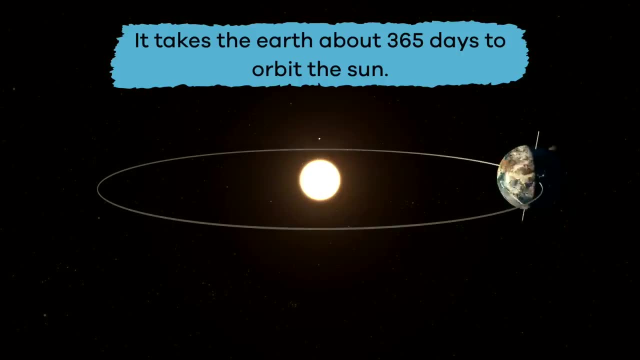 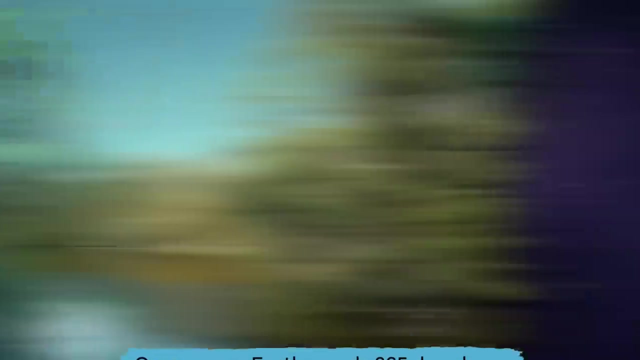 and each planet takes a different amount of time to orbit the Sun. For example, it takes the Earth about 365 days to orbit the Sun. So one year on Earth equals 365 days long. The farther away a planet is from the Sun. the longer it takes to complete its orbit. While the planets are orbiting around the Sun, they are also rotating or spinning. The amount of time it takes for a planet to spin around one time equals the length of one day On Earth. one day equals 24 hours. 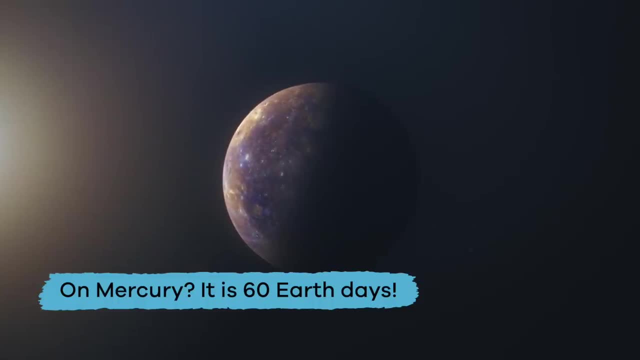 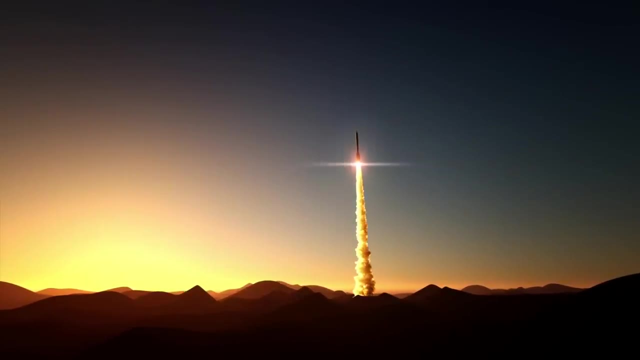 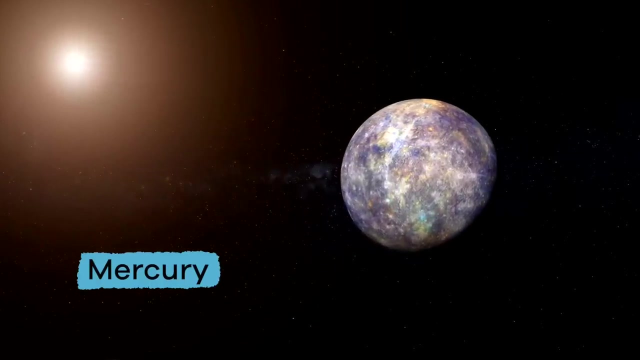 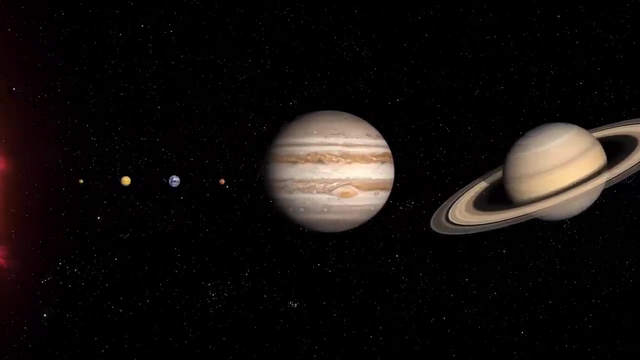 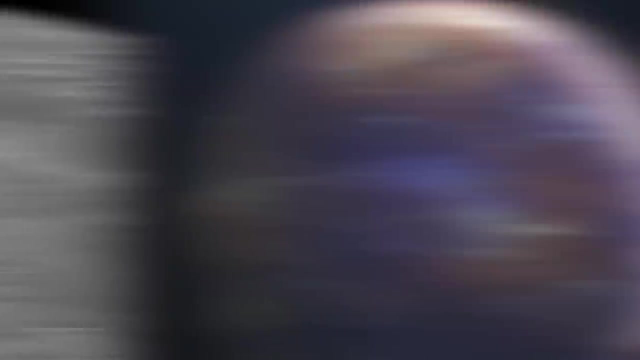 On Mercury. it is 60 Earth days. Let's jump into our spaceship and look at each planet individually so we can learn some more interesting facts. We are going to start with Mercury, which is the planet closest to the Sun. Mercury is the smallest planet in the solar system. It is a rocky planet covered in craters. 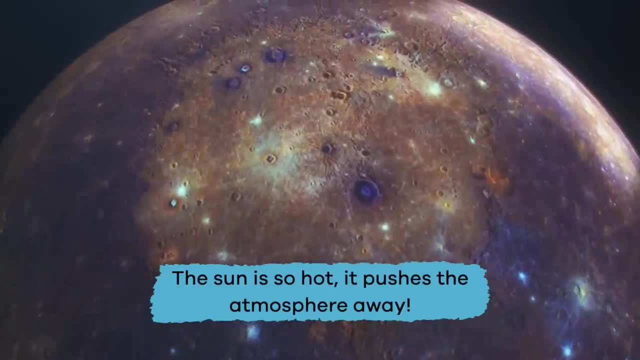 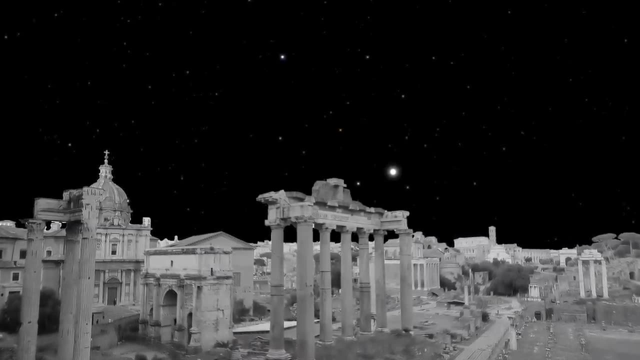 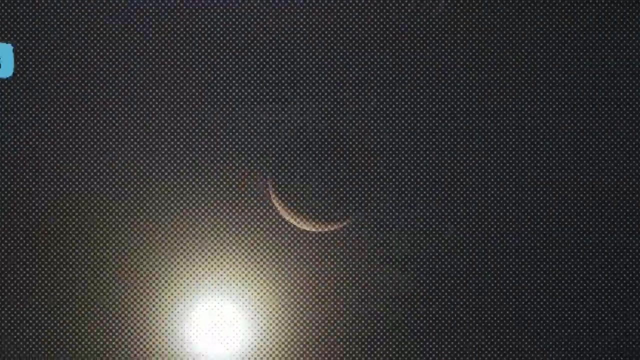 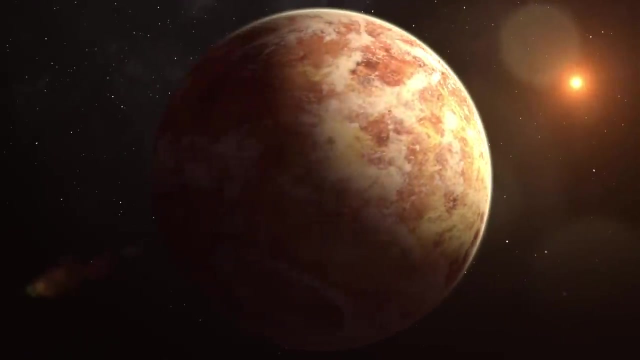 The Sun is so hot it pushes the atmosphere away. It has been known since ancient times because it can be seen without advanced telescopes. Oh, and guess what? Mercury has no moons. Next up is Venus, Similar in size to Earth. it is the hottest planet of them all, with a thick atmosphere. 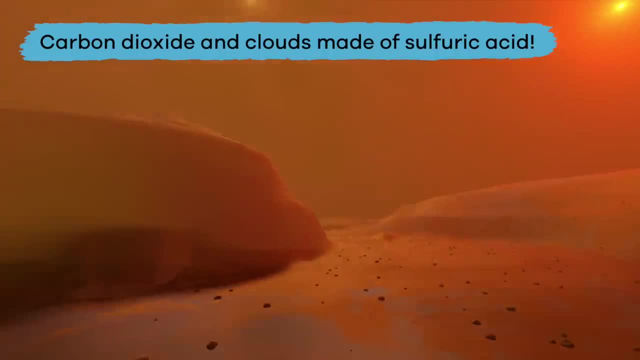 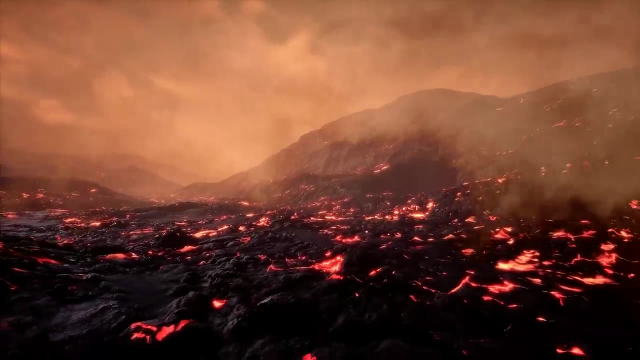 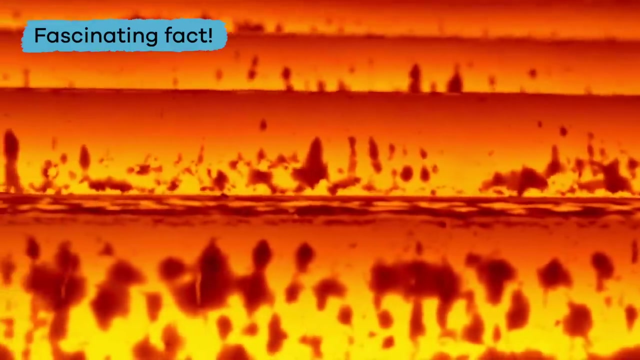 of carbon dioxide and clouds made of sulfuric acid. The rocky planet also has lots of mountains and active volcanoes. Here is a fascinating fact: It is so hot on Venus that metals like lead would not be solid. They would be puddles of liquid. 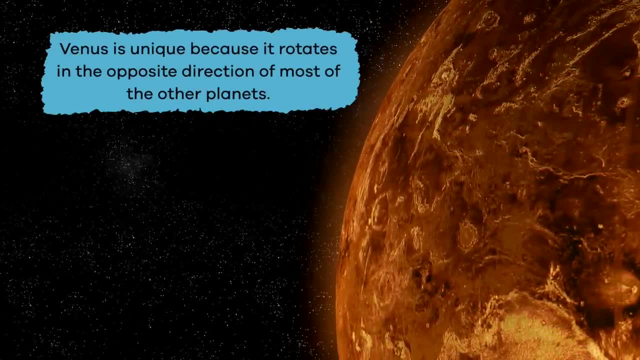 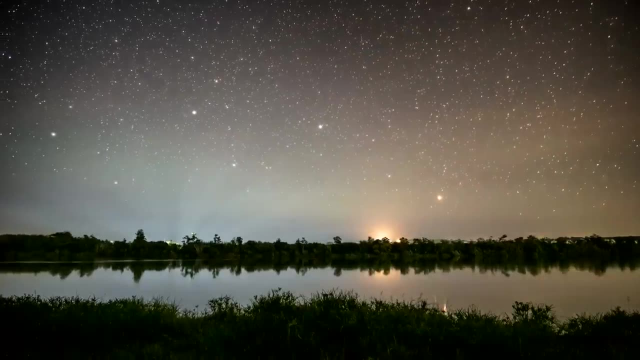 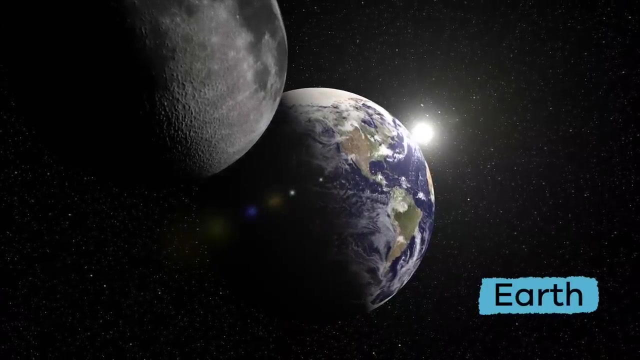 Venus is unique because it rotates in the opposite direction of most of the other planets. It has no moons and can be easily seen in the night sky without a telescope. The Earth is a rocky planet with one moon. It is the only planet in our solar system. 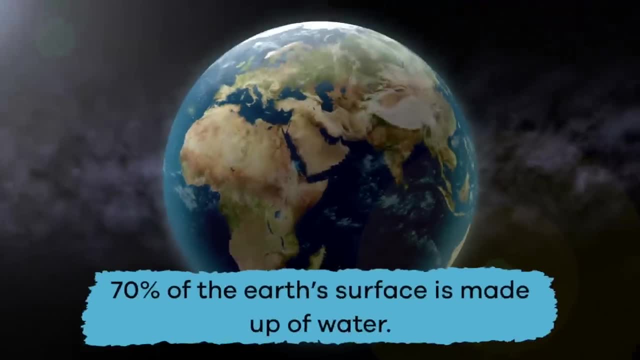 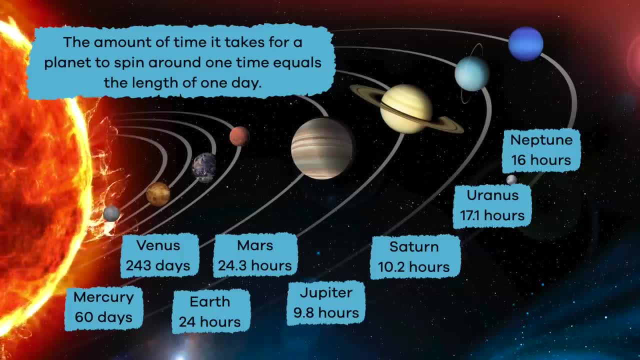 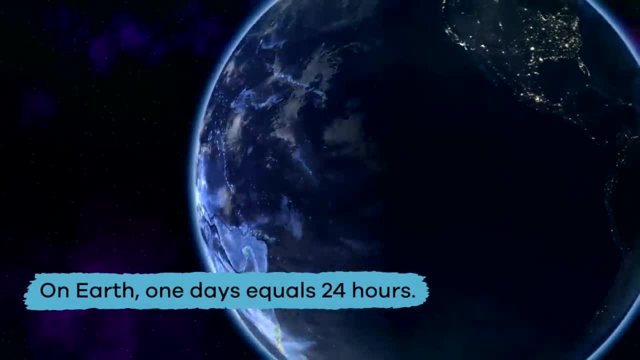 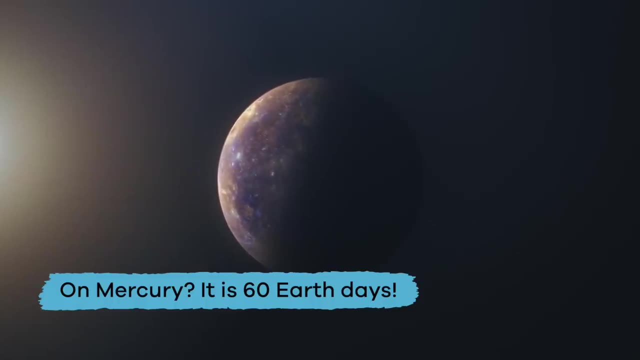 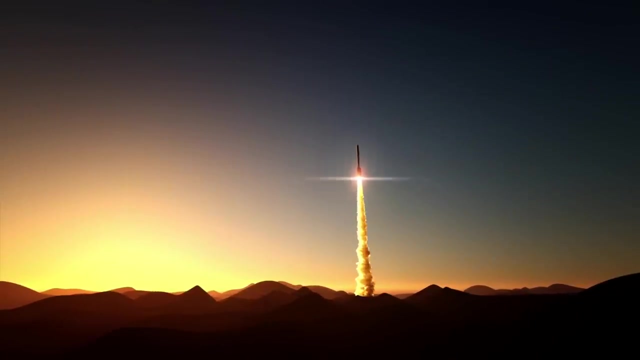 The amount of time it takes for a planet to spin around. one time equals the length of one day On Earth. one day equals 24 hours On Mercury. it is 60 Earth days. Let's jump into our spaceship and look at each planet individually so we can learn some. 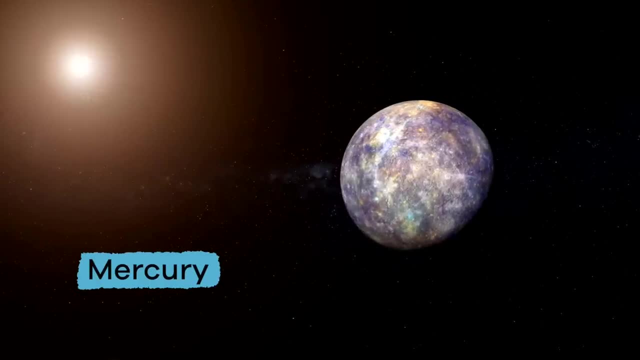 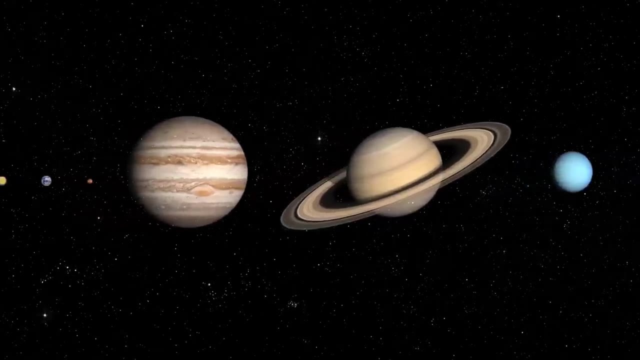 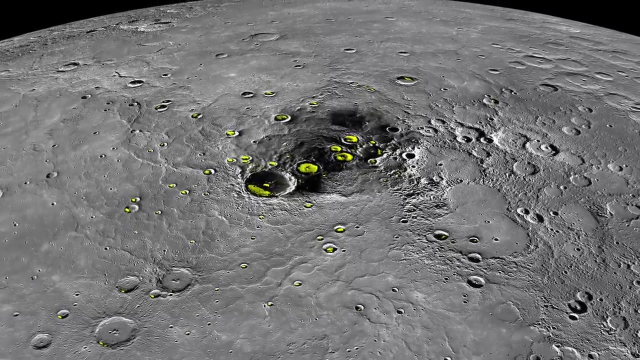 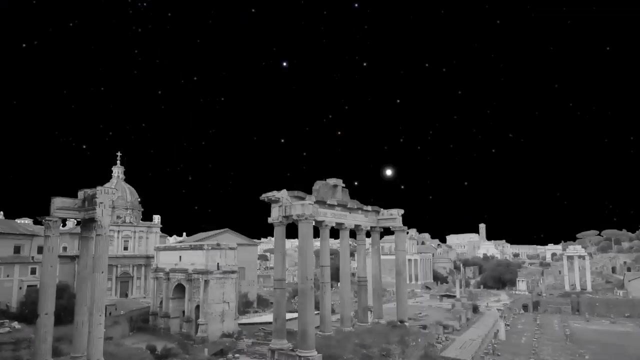 more interesting facts. We are going to start with Mercury, which is the planet closest to the sun. Mercury is the smallest planet in the solar system. It is a rocky planet covered in craters. The sun is so hot it pushes the atmosphere away. It has been known since ancient times. 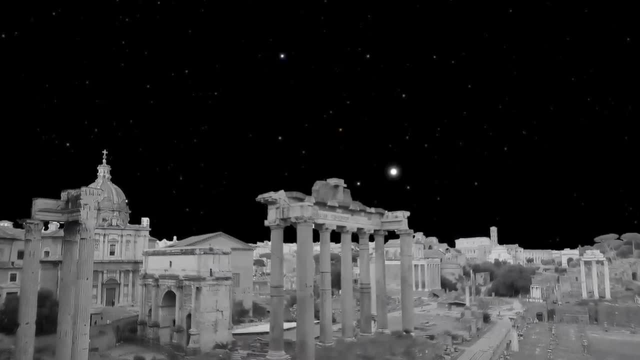 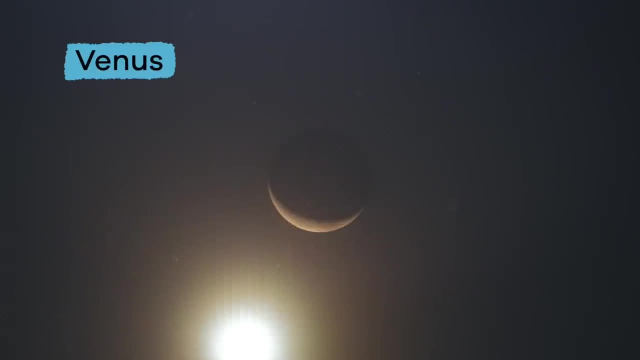 because it can be seen without advanced telescopes. Oh, and guess what? Mercury has no moons. Next up is Venus. Venus is the smallest planet in the solar system. It is the smallest planet in the solar system. It is the smallest planet in the solar system. It is the smallest planet in the solar system. 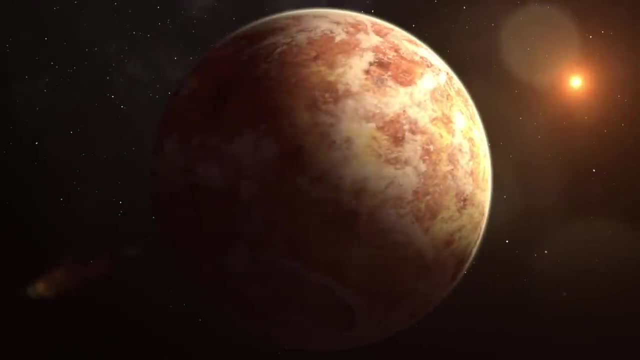 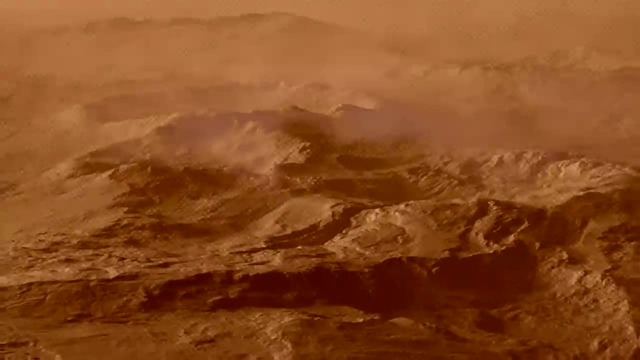 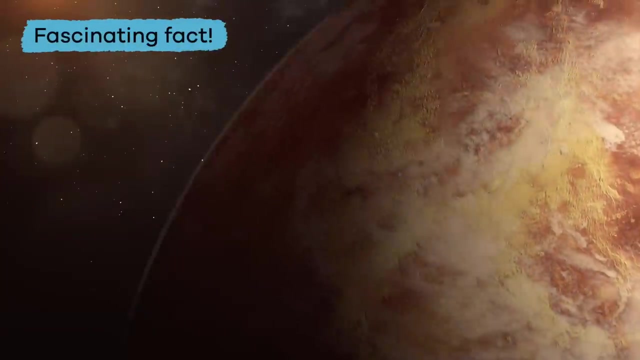 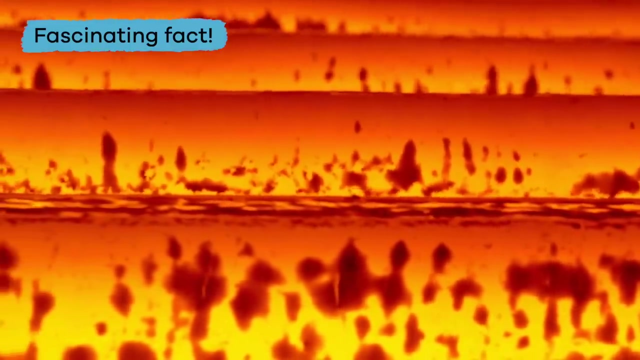 In size to Earth. it is the hottest planet of them all, with a thick atmosphere of carbon dioxide and clouds made of sulfuric acid. The rocky planet also has lots of mountains and active volcanoes. Here is a fascinating fact: It is so hot on Venus that metals like lead would not be solid. 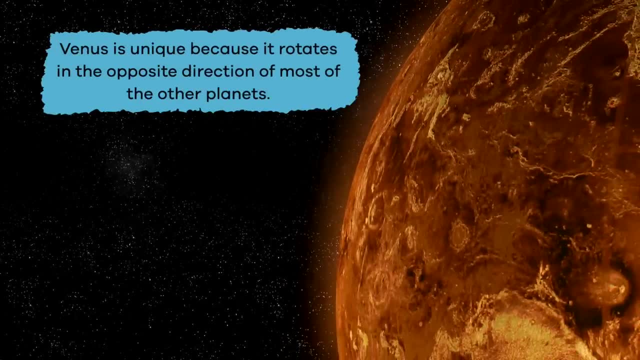 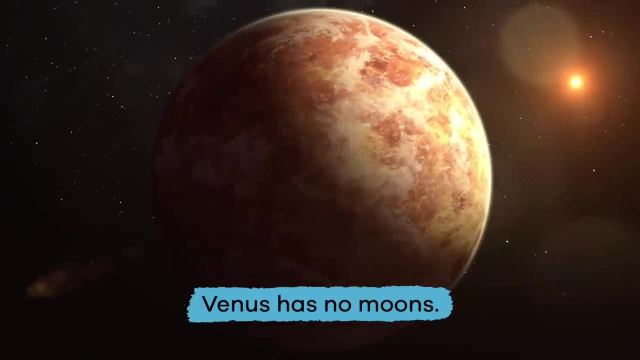 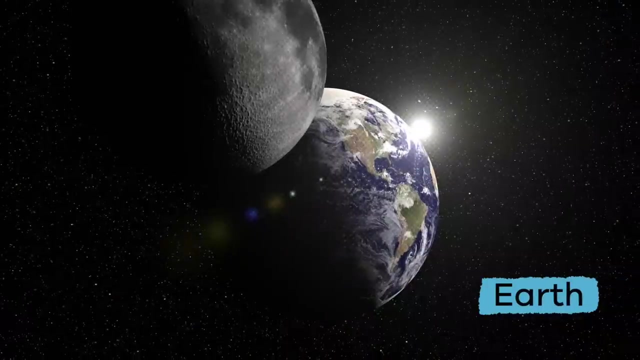 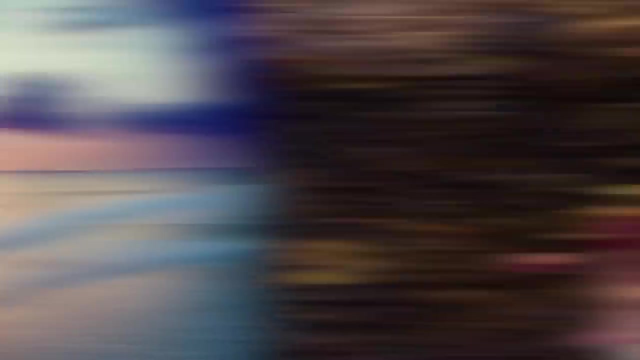 They would be puddles of liquid- is unique because it rotates in the opposite direction of most of the other planets. It has no moons and can be easily seen in the night sky without a telescope. The Earth is a rocky planet with one moon. It is the only planet in our solar system. 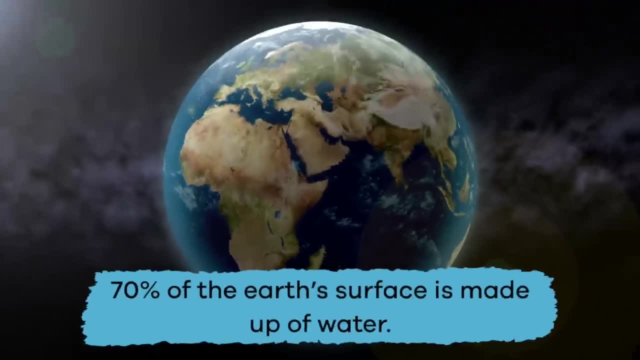 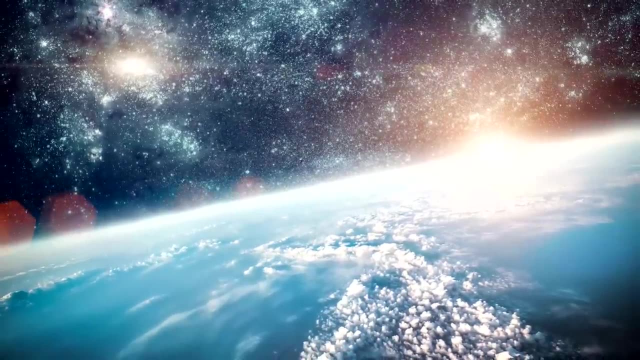 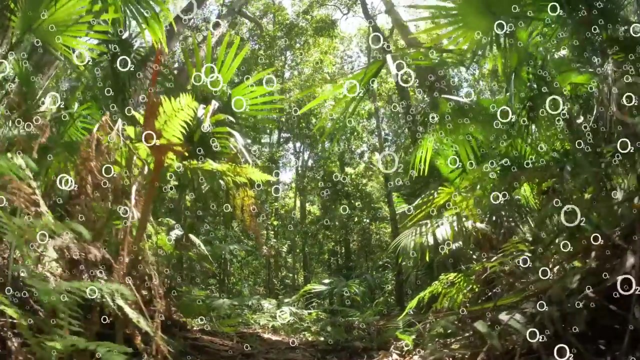 that we know of that supports life. 70% of the Earth's surface is made up of water. The Earth's atmosphere has just the right amount of thickness to protect the planet from the sun and meteorites and provides plenty of oxygen for us to breathe. 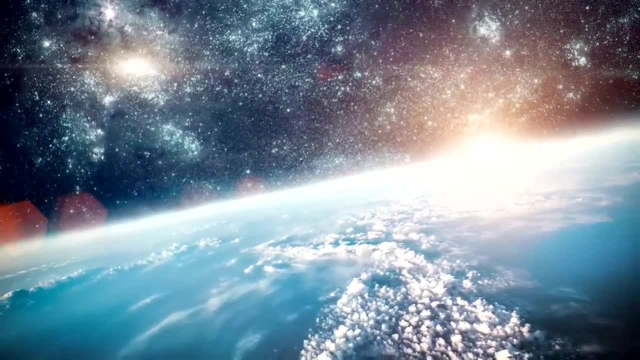 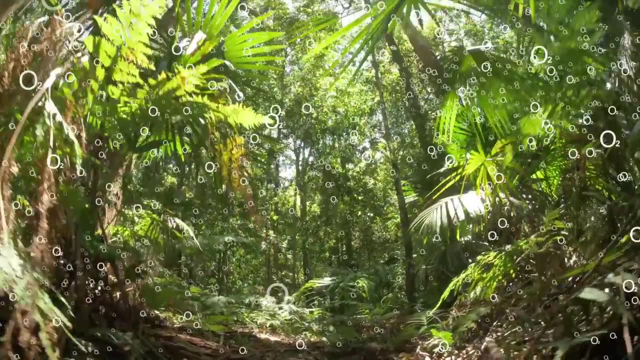 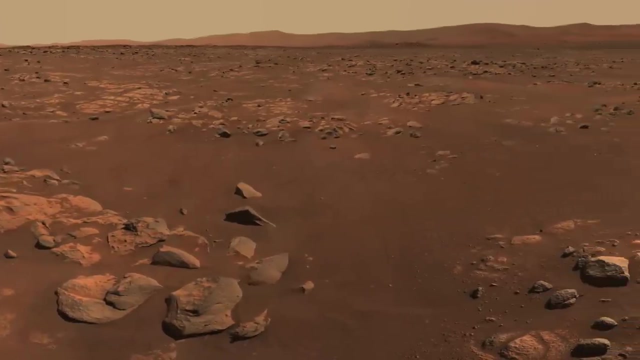 The Earth's atmosphere has just the right amount of thickness to protect the planet from the sun and meteorites and provides plenty of oxygen for us to breathe. Mars, This rocky planet, is a cold desert world with two moons and is about half the size. 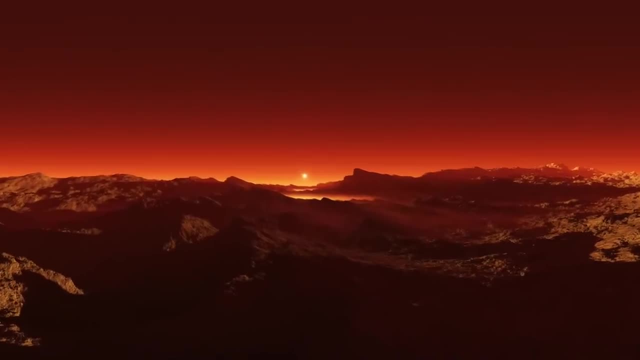 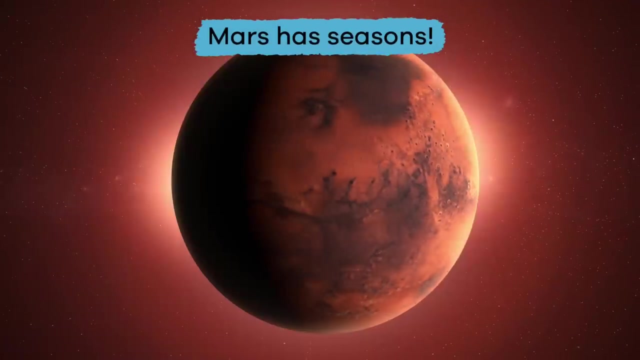 of Earth. Sometimes Mars is called the Red Planet because of its shape. It is a rocky planet and sun-wplin-like Somewhere, and below the temperature is around. the sometime was between 7 and 8 degrees impossible, so a vast amount of the more terrible weather can green up from below. 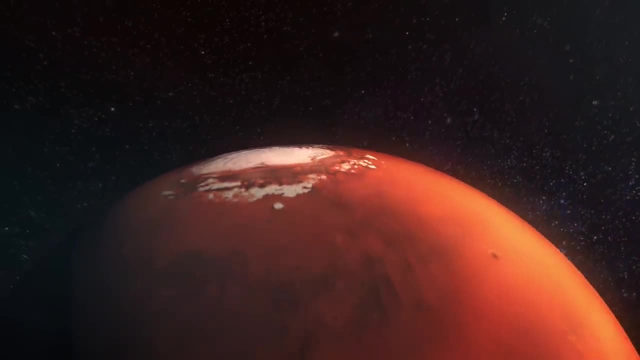 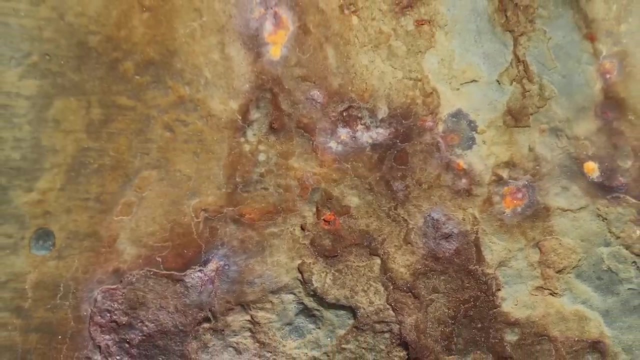 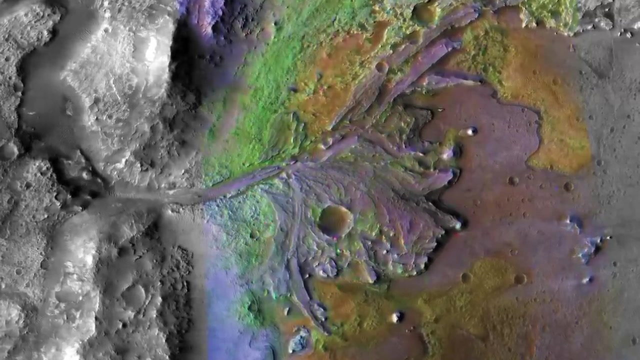 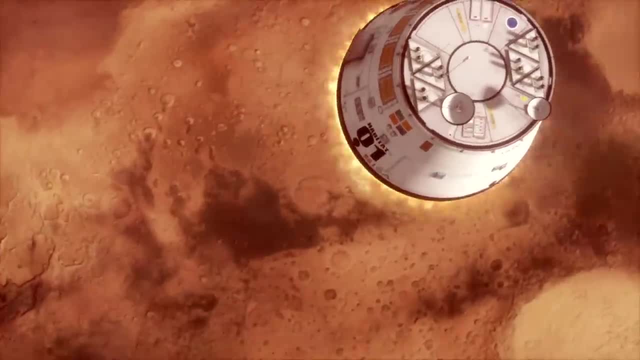 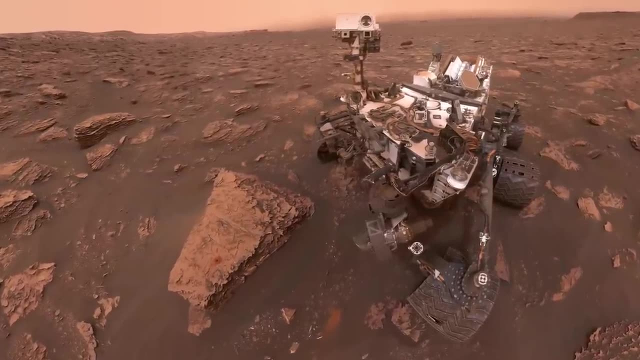 06 07 07. 07 07. 08 07 07 07. in order to see if the planet could sustain life in the future, and have sent rovers to explore the planet's surface. Here's an interesting fact: Mars is the only planet where we have sent rovers. 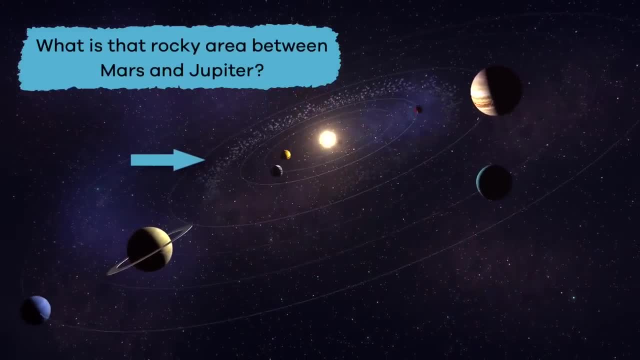 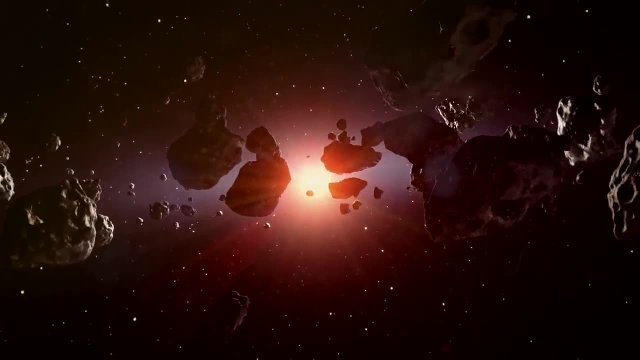 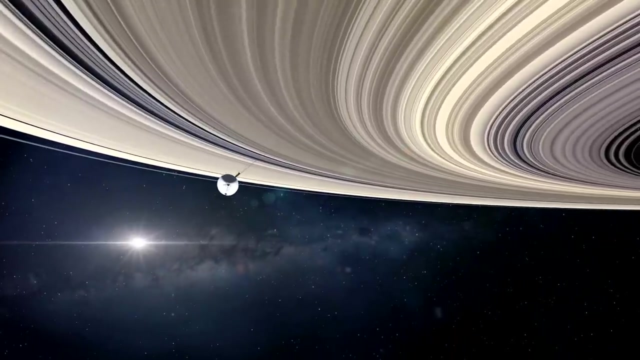 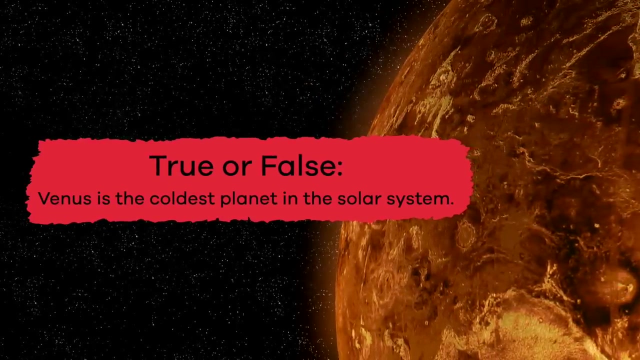 What is that rocky area between Mars and Jupiter? It is the asteroid belt which contains rocky, irregularly shaped bodies called- you guessed it- asteroids. While we pass through it, let's take a minute to review True or false. Venus is the coldest planet in the solar system. 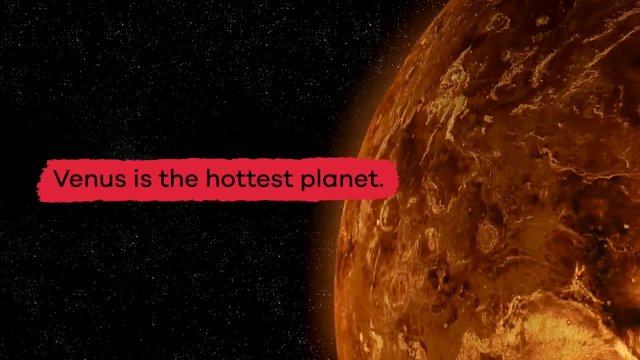 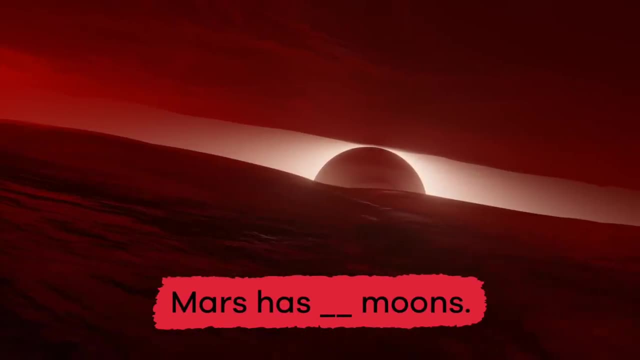 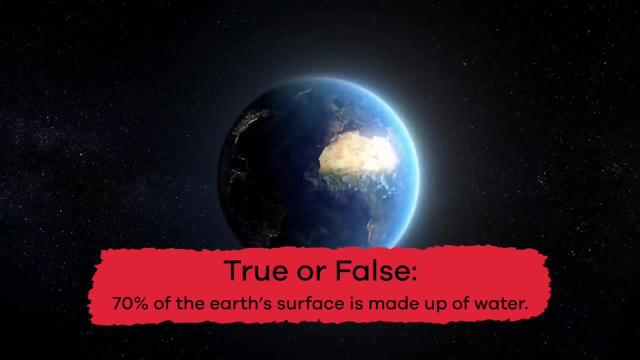 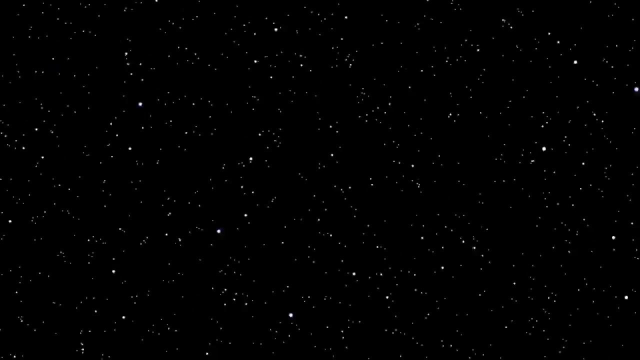 False: Venus is the hottest planet. Fill in the blank: Mars has blank moons, Two moons, True, False. True or false. 70% of Earth's surface is made up of water. True, Great job. Now let's head to Jupiter. 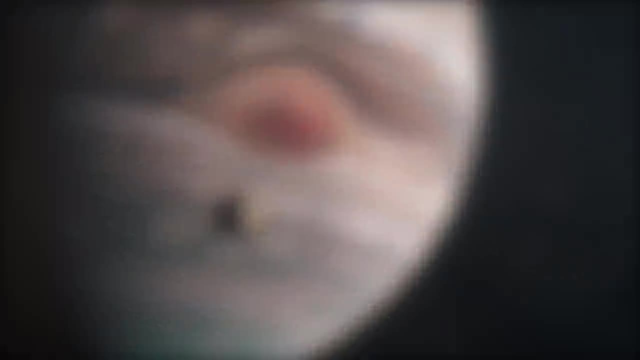 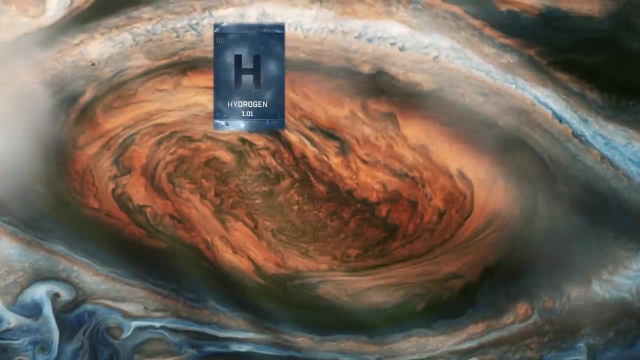 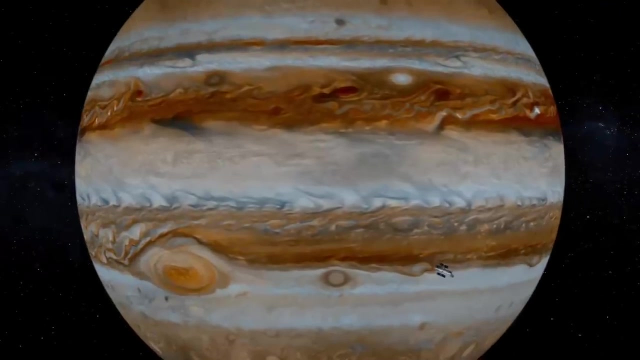 Jupiter is the first gas giant planet we are visiting, which means we definitely could not stand on its surface, because it is made up of hydrogen and helium. It is our solar system's biggest planet And you might be familiar with this huge red eye. 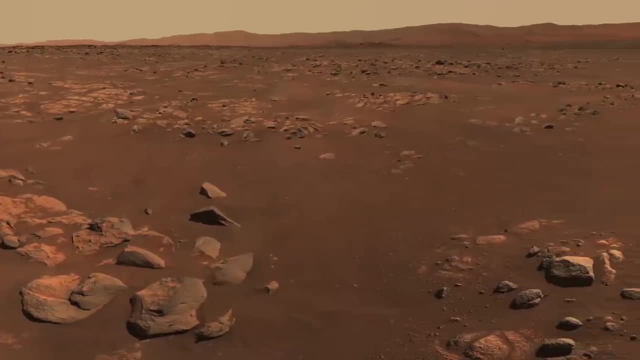 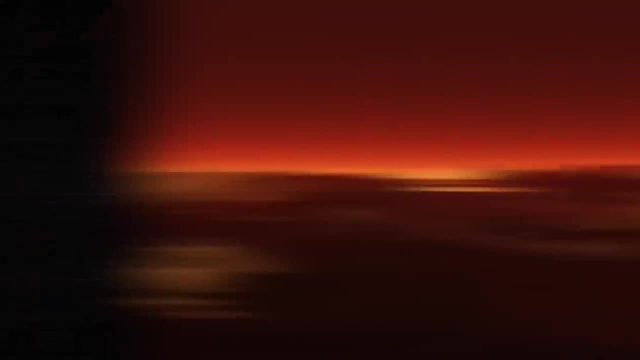 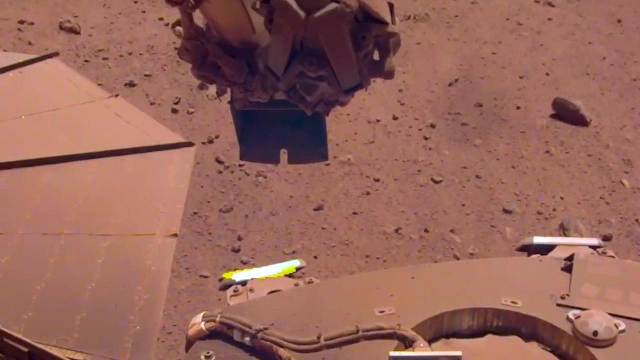 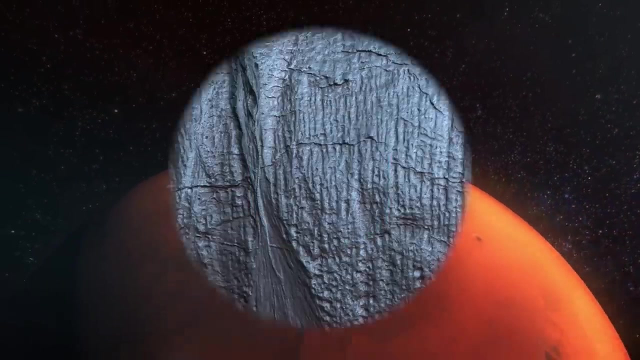 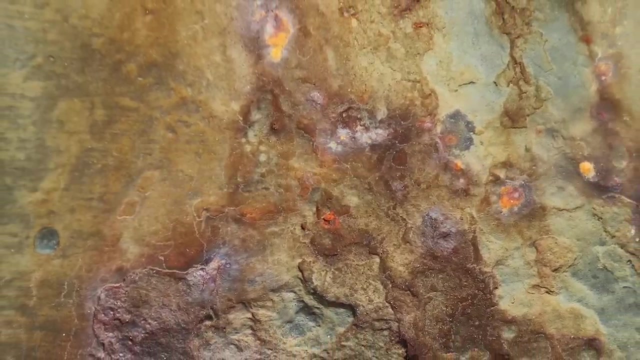 Mars. This rocky planet, is a cold desert world with two moons and is about half the size of Earth. Sometimes Mars is called the Red Planet because of rusty eyes. Mars has seasons and at one time probably had flowing water. There are signs of ancient floods, but now the only water on the planet is found in icy. 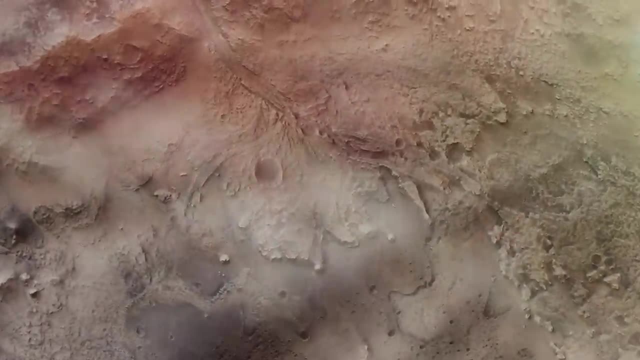 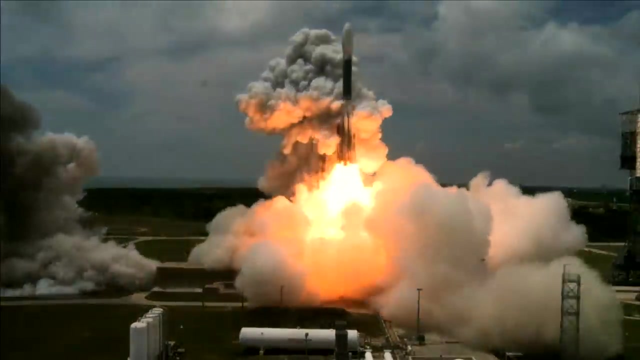 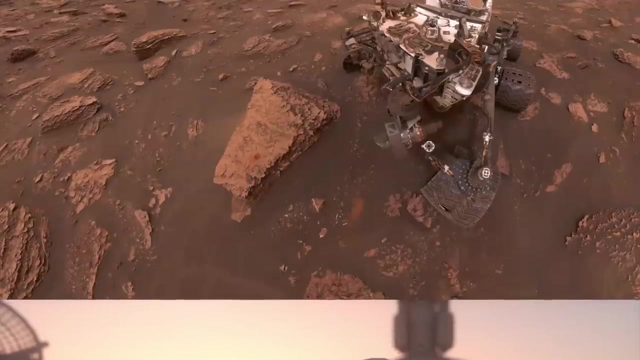 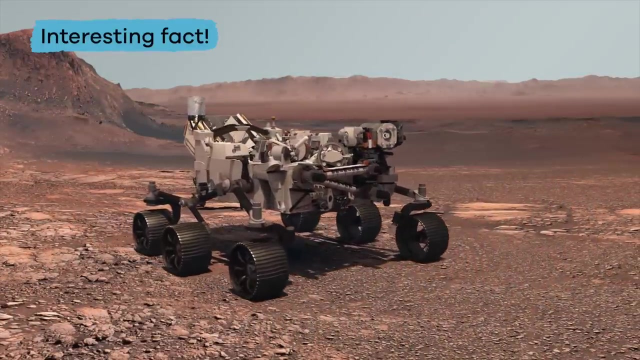 soil and thin clouds. There may also be liquid salty water in the ground too. Scientists are super interested to study Mars in order to see if the planet could sustain life in the future and have sent rovers to explore the planet's surface. Here's an interesting fact: Mars is the only planet where we have sent rovers. 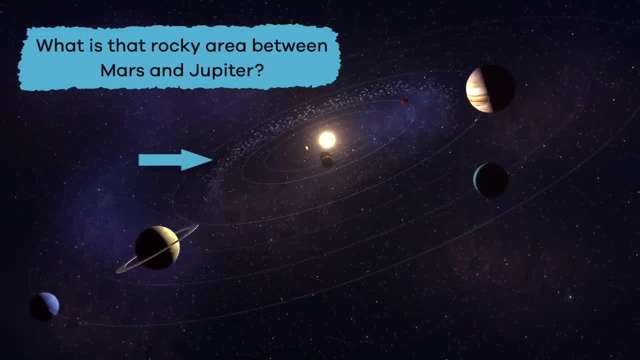 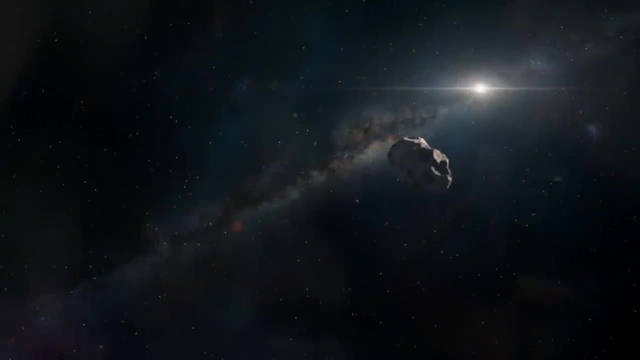 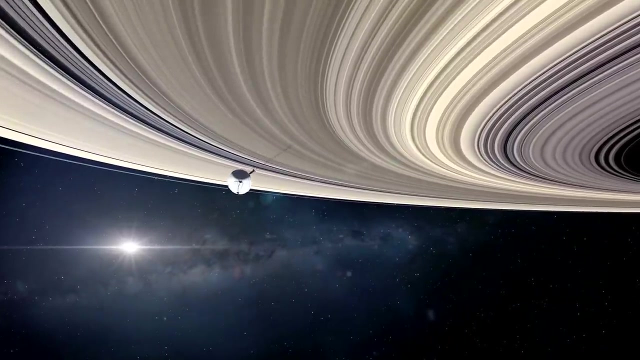 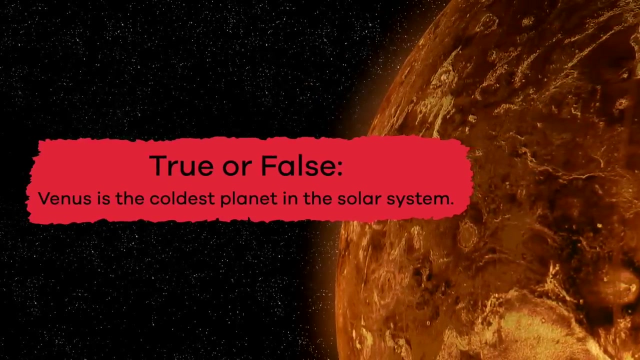 What is that rocky area between Mars and Jupiter? It is the asteroid belt which contains rocky, irregularly shaped bodies called- you guessed it- asteroids. While we pass through it, let's take a minute to review True or false. Venus is the coldest planet in the solar system. 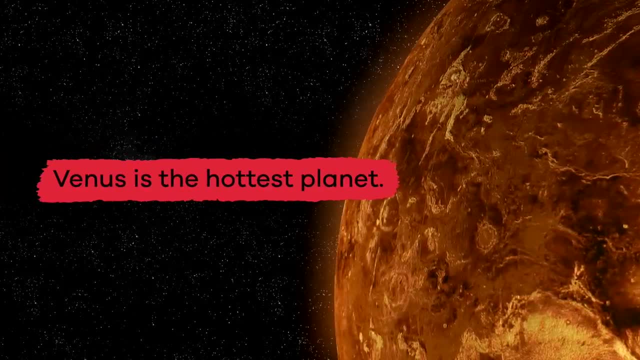 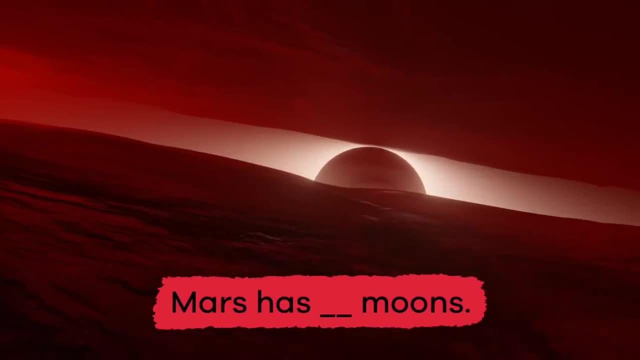 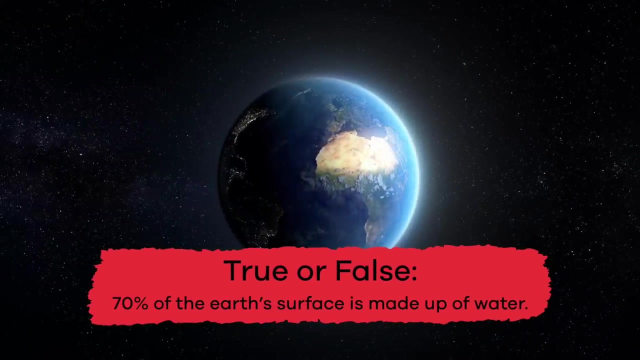 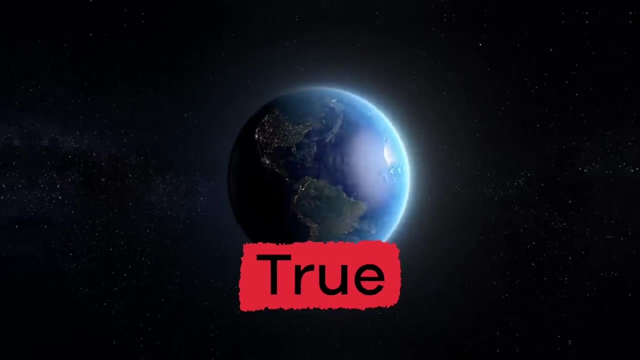 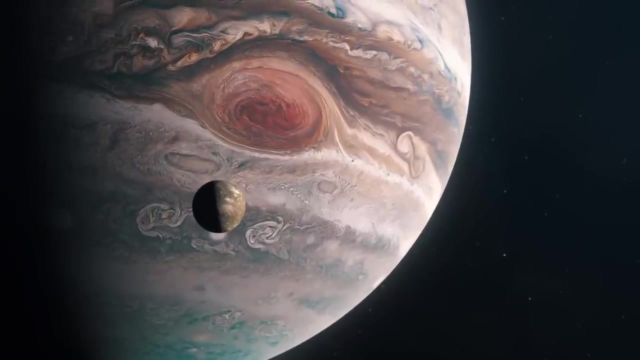 False: Venus is the hottest planet. Fill in the blank: Mars has ______ moons, Two moons. True or false? 70% of Earth's surface is made up of water. True, Great job. Now let's head to Jupiter. Jupiter is the first gas giant planet we are visiting, which means we definitely could. 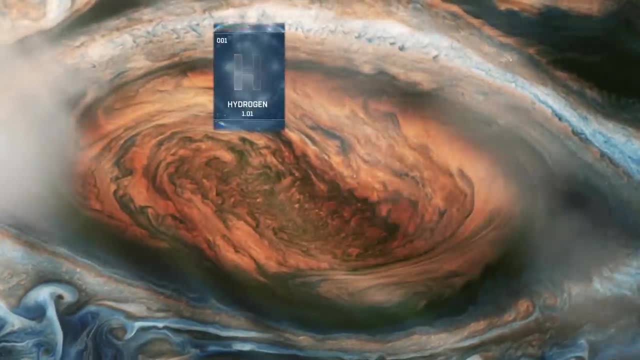 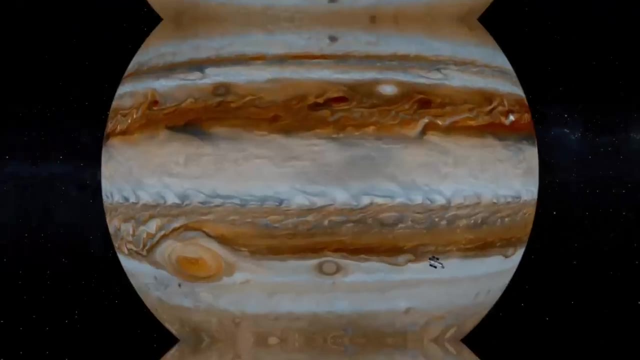 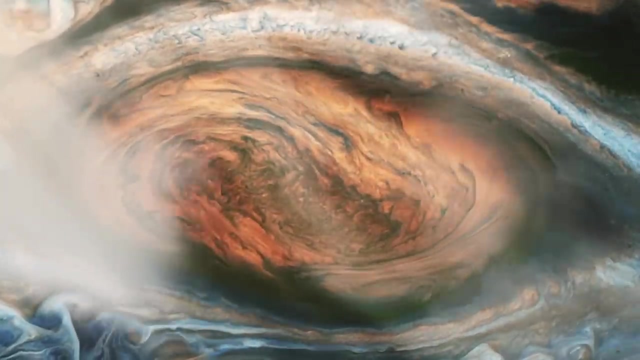 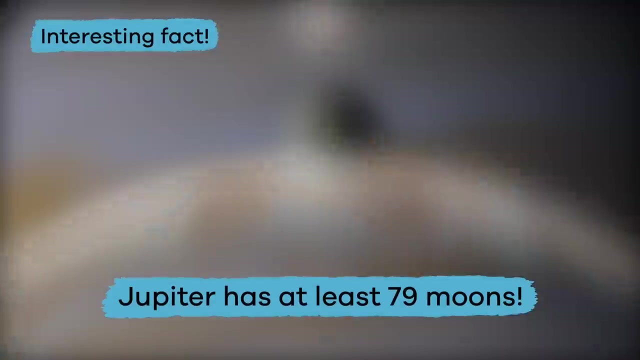 not stand on its surface, because it is made up of hydrogen and helium. It is our solar system's biggest planet And you might be familiar with this huge red eye, which is actually the site of huge, continuous storms. Here is an interesting fact: Jupiter has at least 79 moons, the most of all the planets. 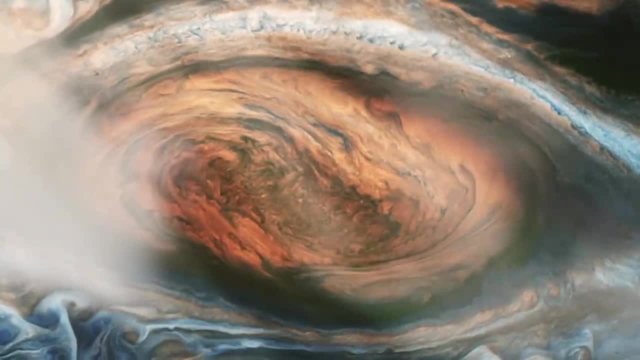 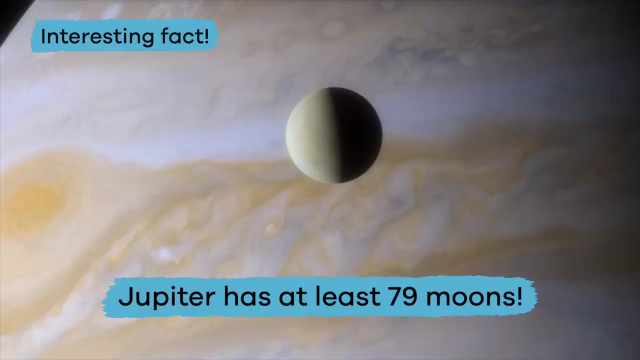 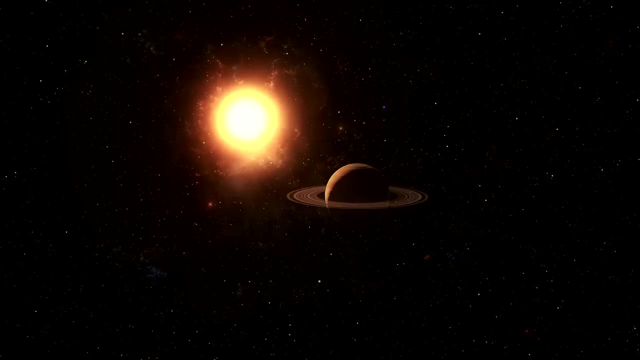 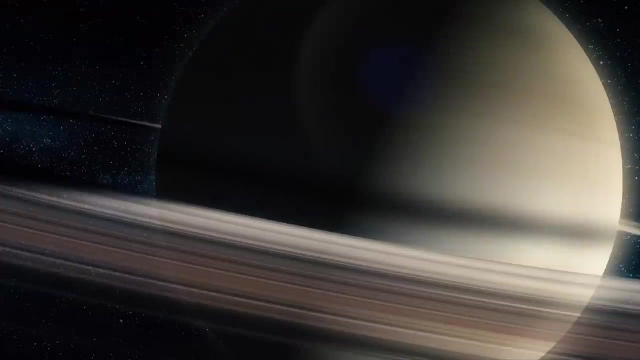 which is actually the site of huge, continuous storms. Here is an interesting fact: Jupiter has at least 79 moons- the most of all the planets- Plus it has rings, but they are very hard to see. Saturn Also, a gas giant made of hydrogen and helium. 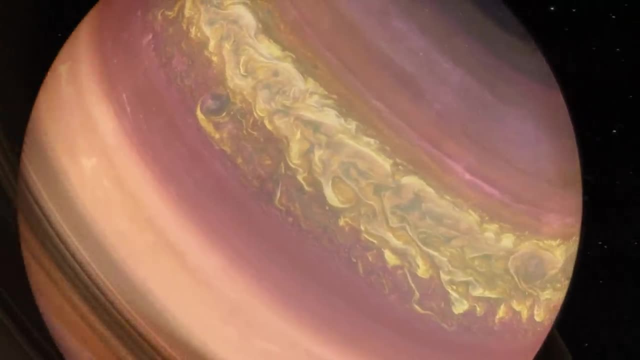 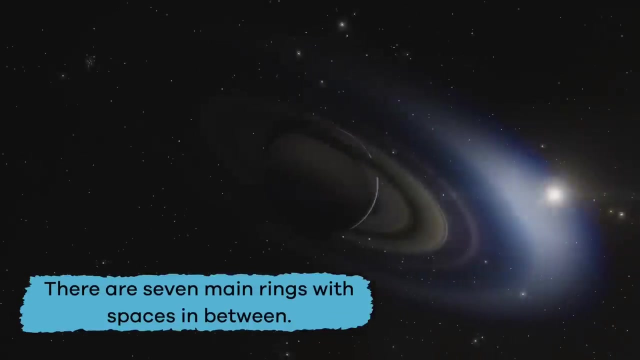 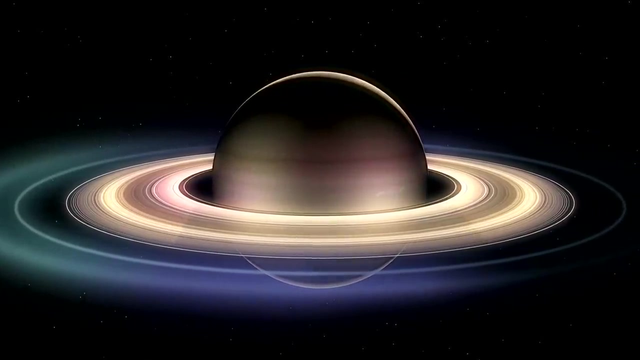 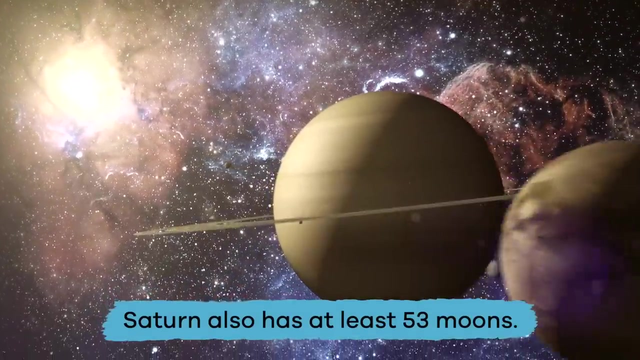 Saturn has a thick atmosphere and is probably best known for its beautiful, distinct rings. There are seven main rings, with spaces in between, and each ring is made up of groups of tiny ringlets made of ice chunks and rocks. Also, Saturn has at least 53 moons. 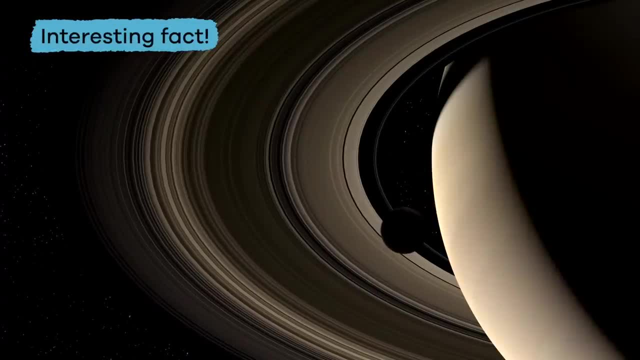 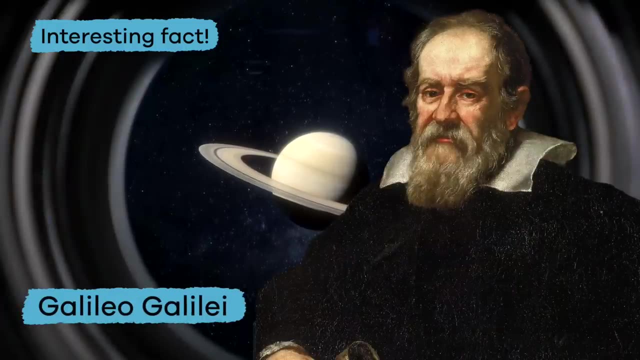 Want to know an interesting fact about Saturn. The famous astronomer Galileo saw Saturn through a telescope way back in the 1600s. Uranus Discovered in 1782 by a British astronomer named William Herschel. Uranus is an ice giant. 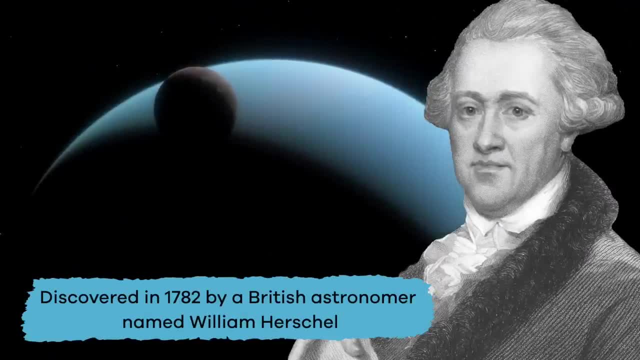 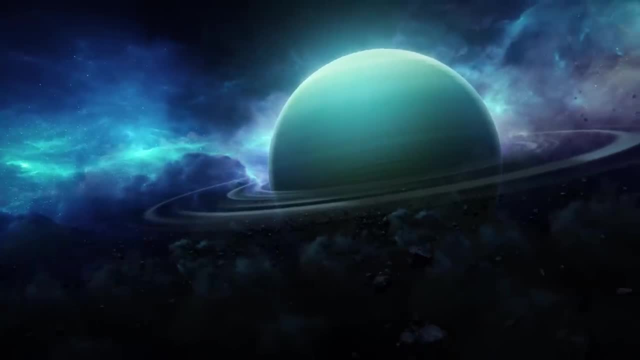 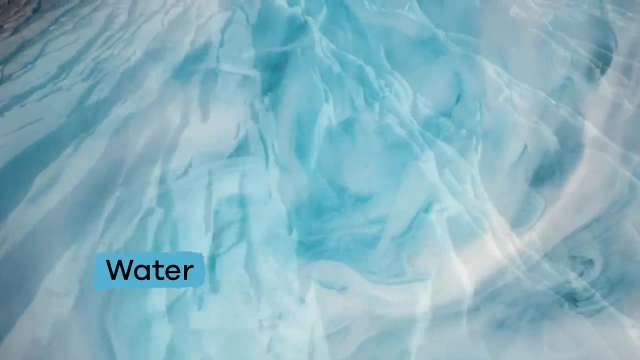 which means that it is mostly made of flowing icy water. Uranus is also known as the ice giant because it is the largest ice giant in the world. Uranus is the largest ice giant made of flowing icy materials- things like water, methane. 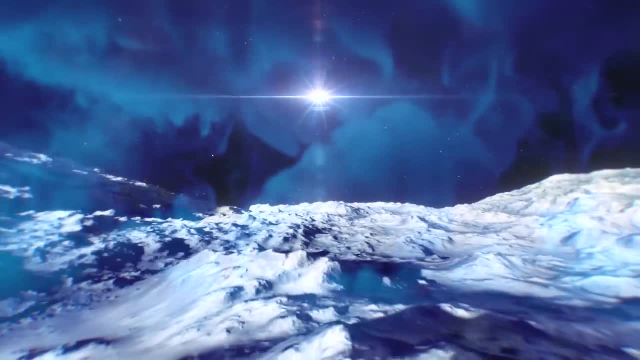 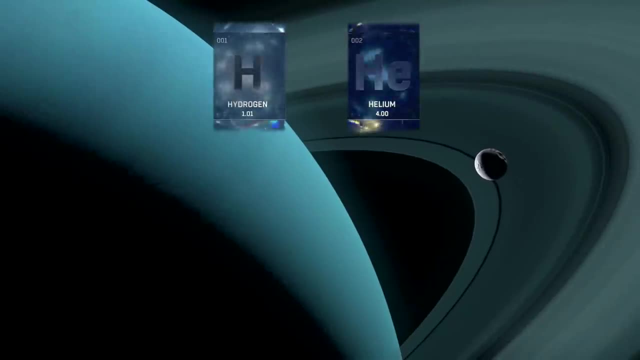 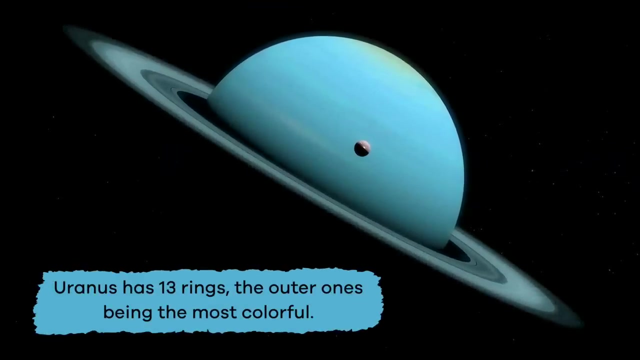 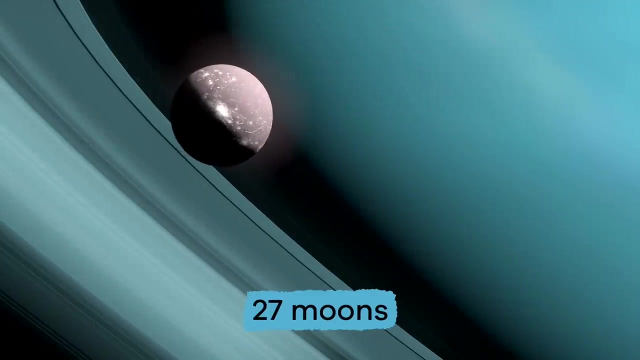 and ammonia fluids that surround a small rocky center. Its atmosphere is thick with hydrogen and helium, but also methane, which is what makes it blue in color. Uranus has 13 rings, the outer ones being the most colorful, and 27 moons. 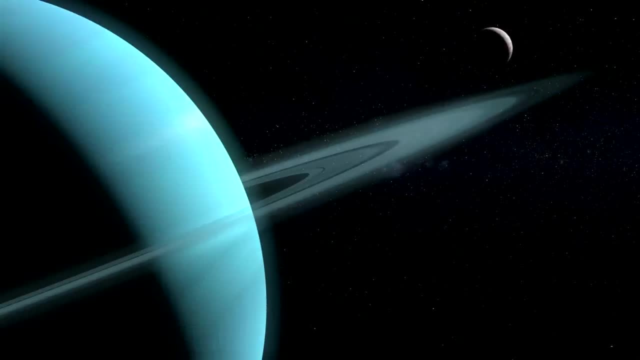 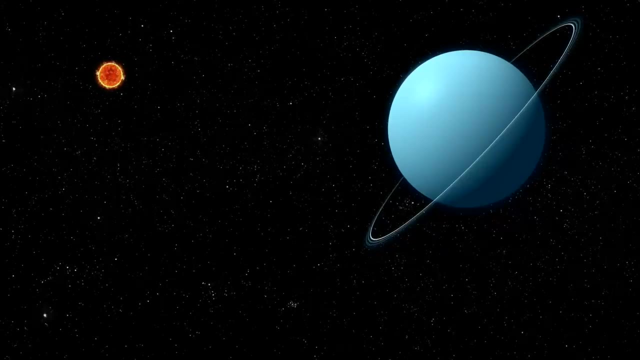 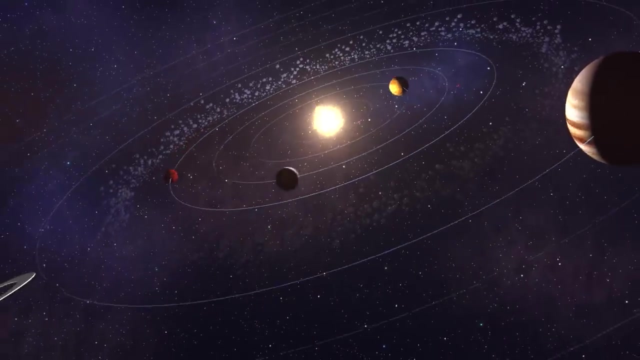 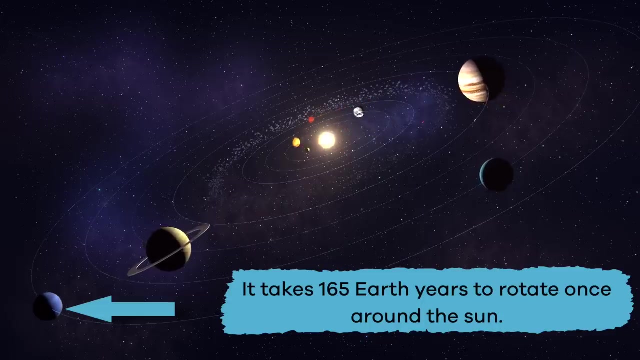 Like Venus, Uranus rotates in the opposite direction And, unlike any other planet, it rotates on its side. Last but not least is Neptune. Neptune is the farthest planet away and it takes 165 Earth years to rotate once around the Sun. 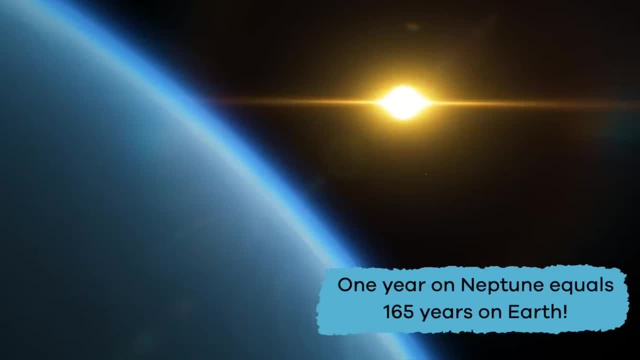 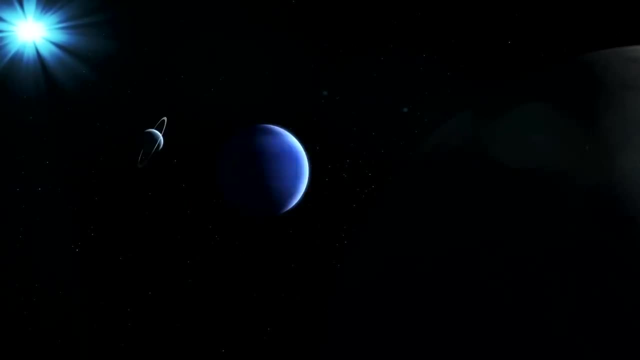 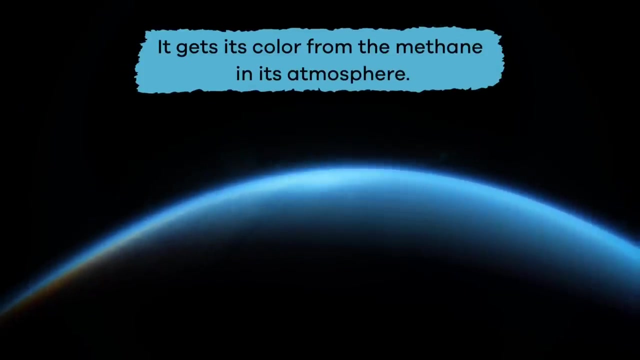 which means that one year on Neptune equals 165 years on Earth. Neptune is an ice giant, like Uranus, And like Uranus, it gets its color from the methane in its atmosphere. Neptune is made of a thick fog of water- ammonia. 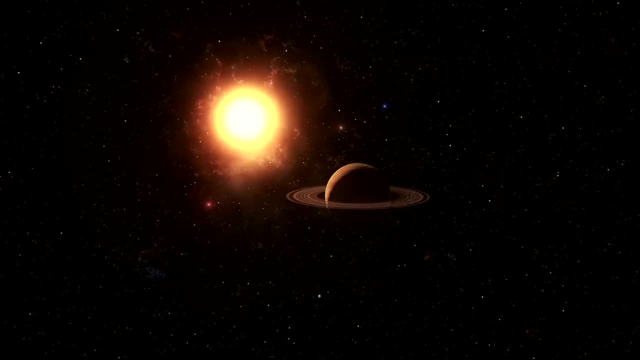 Plus, it has rings, but they are very hard to see. Saturn is also a gas giant. It has a huge red eye and a huge continuous storm. Here is an interesting fact: Jupiter has at least 79 moons, the most of all the planets. 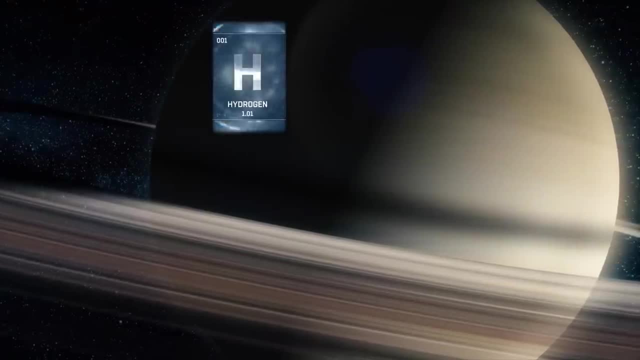 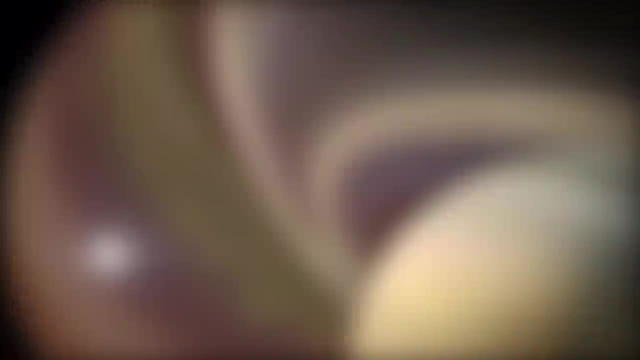 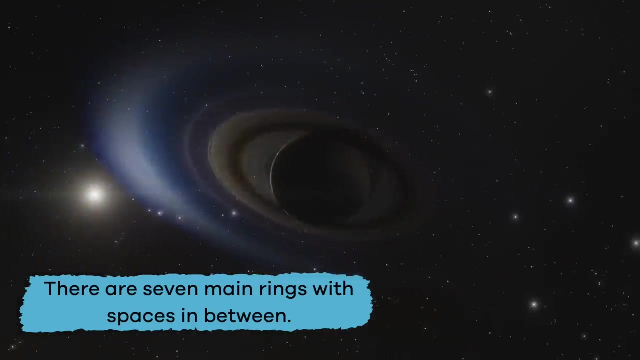 Plus, it has rings, but they are very hard to see, Also a gas giant made of hydrogen and helium. Saturn has a thick atmosphere and is probably best known for its beautiful, distinct rings. There are seven main rings with spaces in between, and each ring is made up of groups. 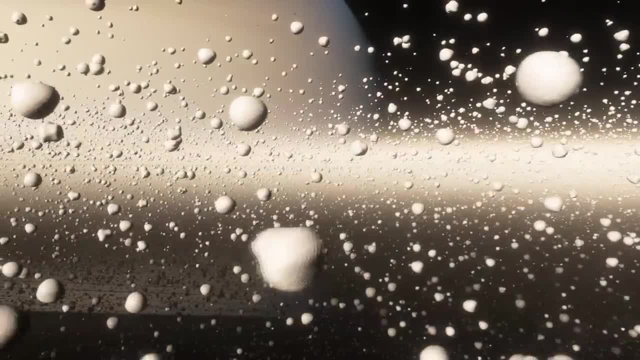 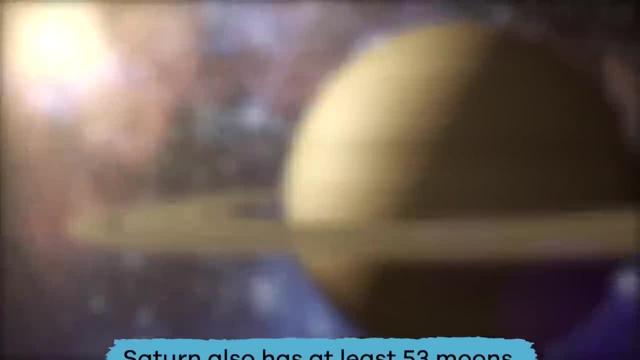 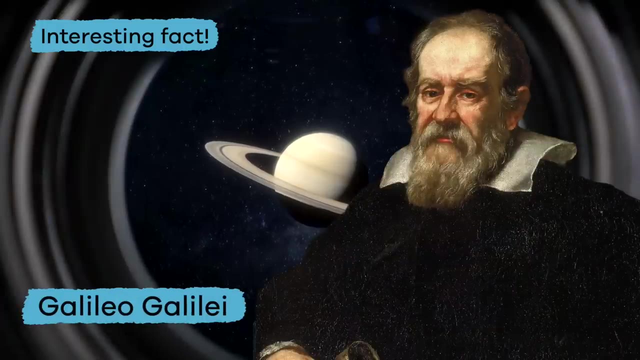 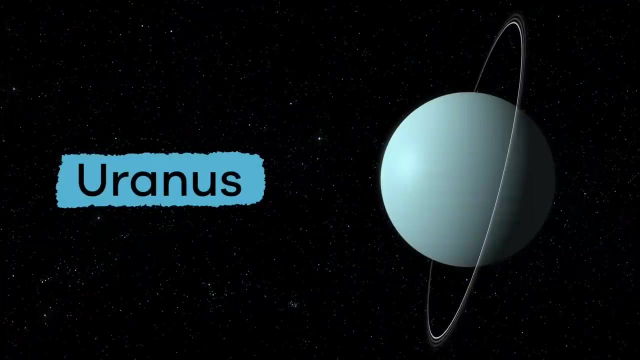 of tiny ringlets made of ice chunks and rocks. Also, Saturn has at least 53 moons. Want to know an interesting fact about Saturn? The famous astronomer Galileo saw Saturn through a telescope way back in the 1600s. Uranus Discovered in 1782 by a British. 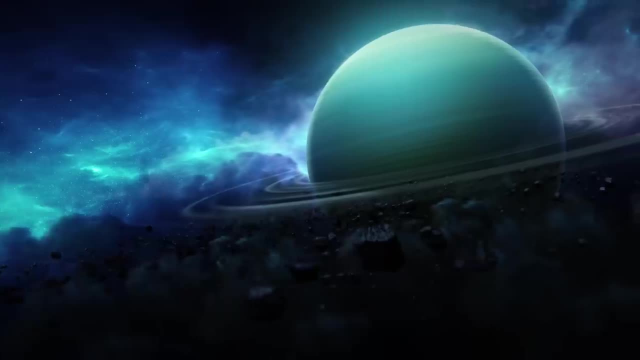 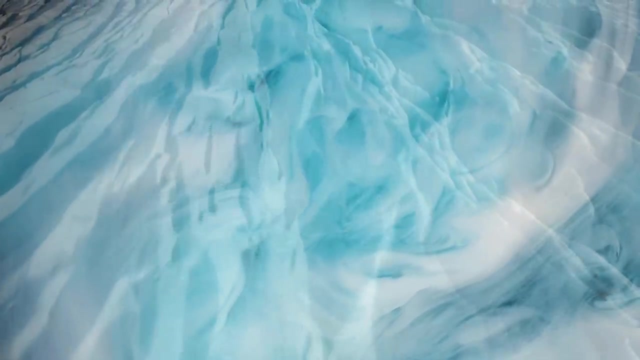 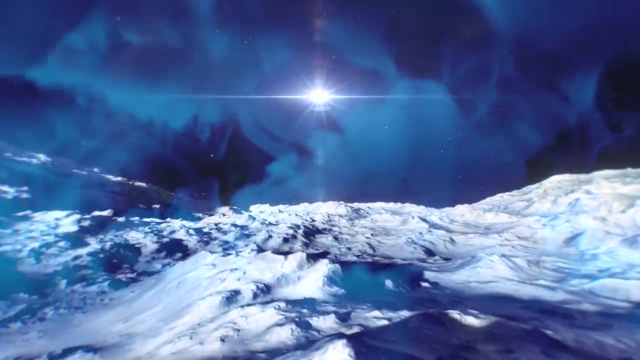 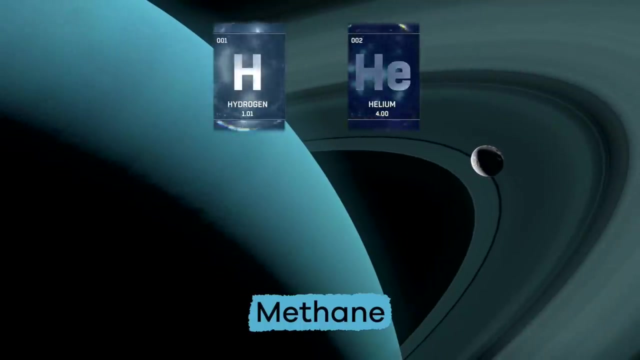 astronomer named William Herschel. Uranus is an ice giant, which means that it is mostly made of flowing icy materials, Things like water, methane and ammonia- fluids that surround a small rocky center. Its atmosphere is thick with hydrogen and helium, but also methane. 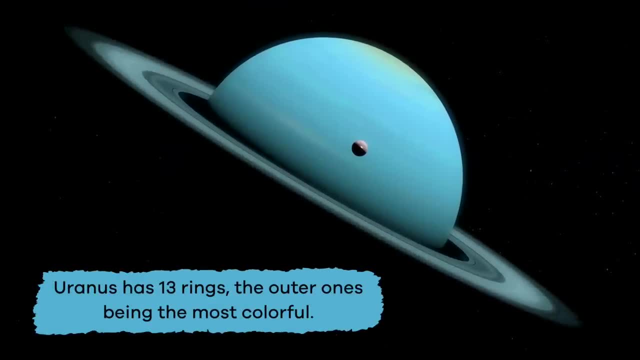 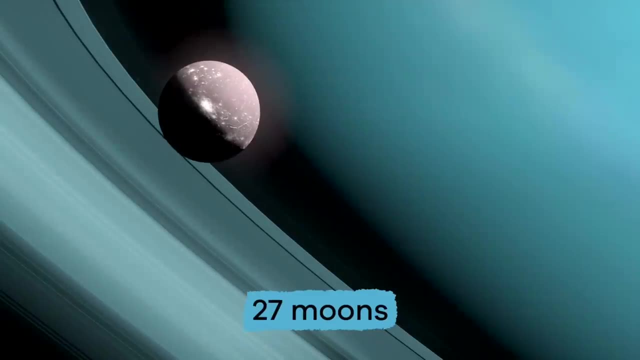 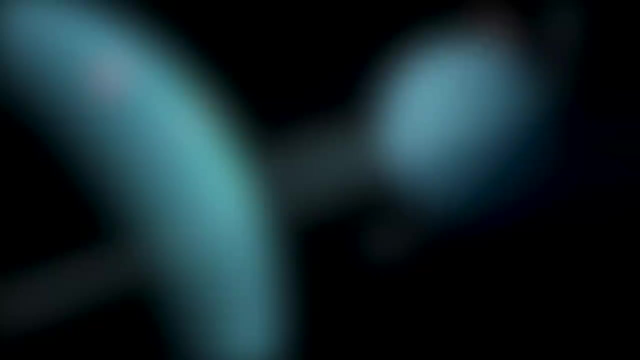 which is what makes it blue in color. Uranus has 13 rings, the outer ones being the most colorful, and 27 moons. Like Venus, Uranus rotates in the opposite direction and, unlike any other planet, it rotates on its side. 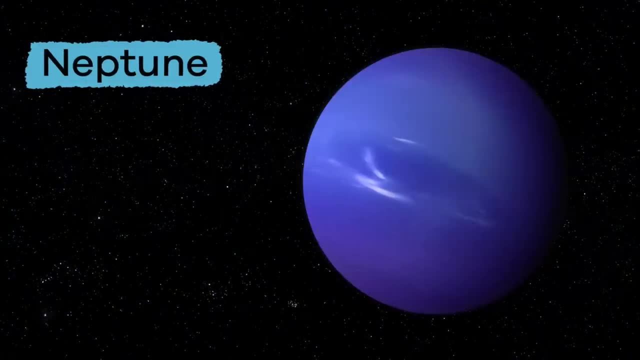 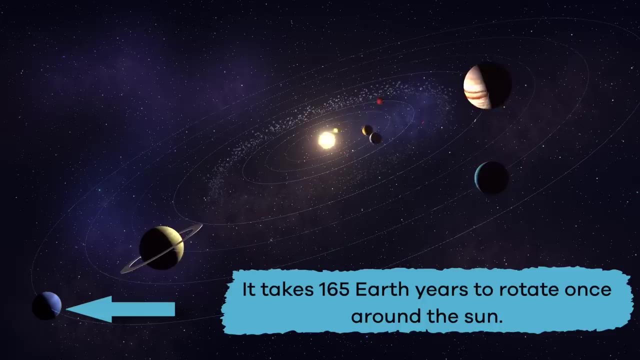 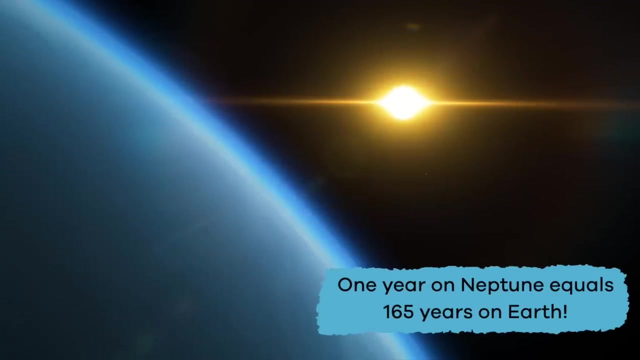 Last but not least is Neptune. Neptune is the farthest planet away and it takes the longest time to reach the surface of the Earth. This means that it takes 165 years to rotate once around the sun, Which means that one year on Neptune equals 165 years on Earth.